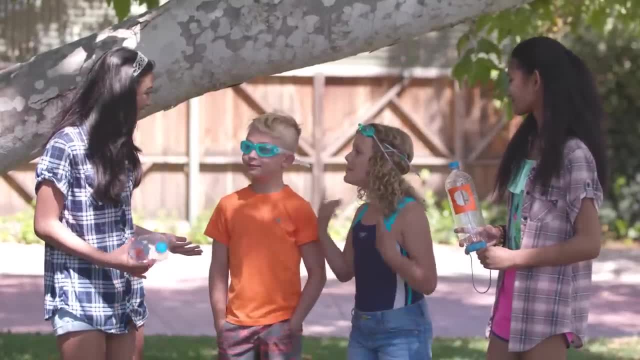 You guys look really hot, Want to get wet? I am. I am dying of heat. Okay, first thing, have your friends put on their goggles, Then place on their headbands So that the bottle faces out like this, And then have your other two people use the squirt guns to see who can get more water. 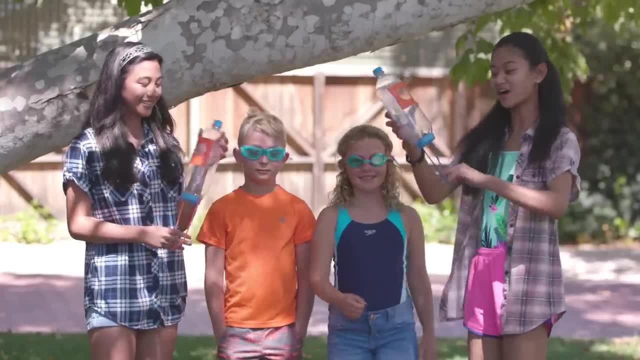 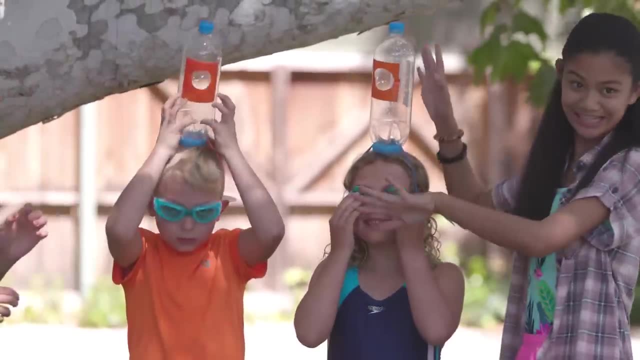 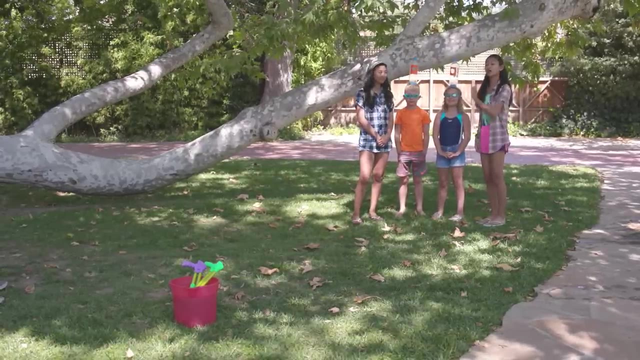 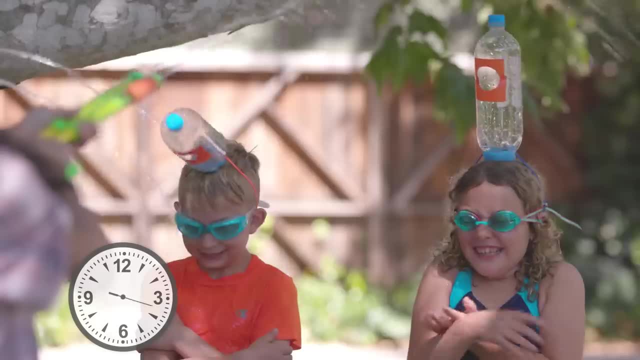 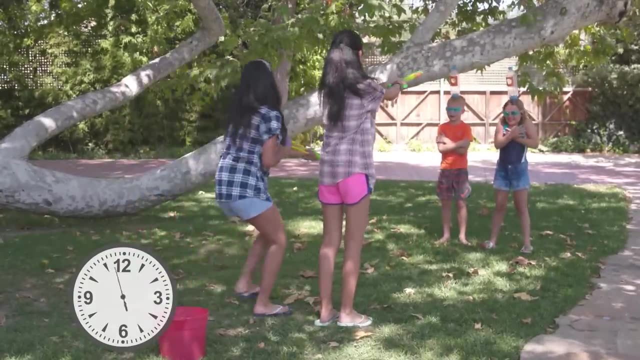 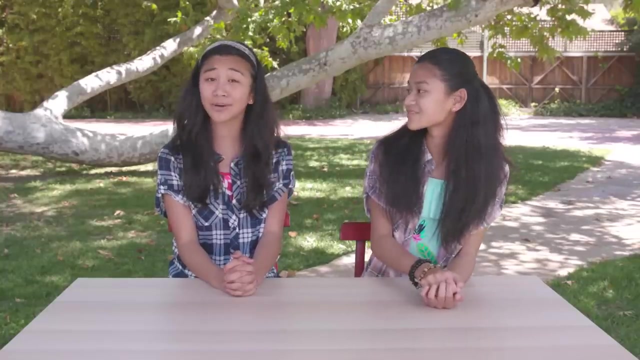 No, No, No, Whoa. Oh my gosh, I am thirsty. It is so hard, I will go higher. okay, I won. Yay, I am close And I don't feel like I am going to pass out anymore. 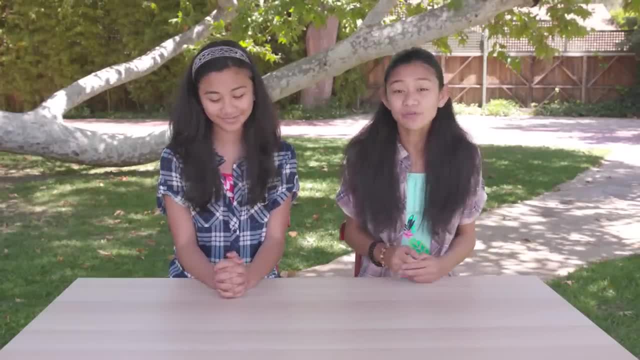 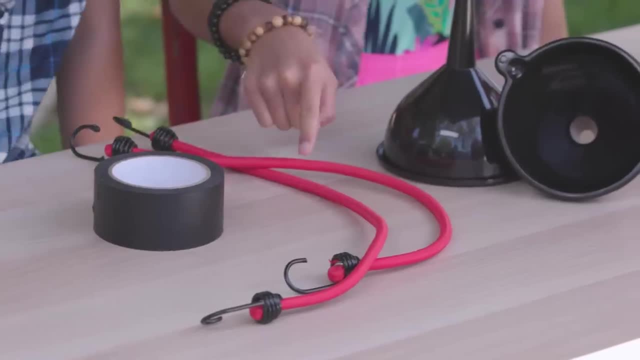 So I win too. Well, then help me with this next hack, A super fun game we can all play together: My Water Balloon Slingshot. For this hack, you will need Tape, Two bungee cords, two funnels that are exactly the same size and water balloons. 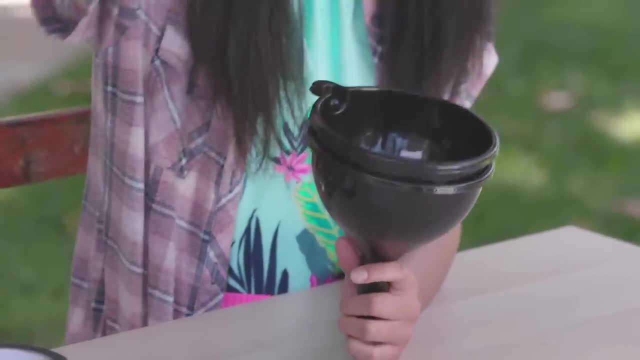 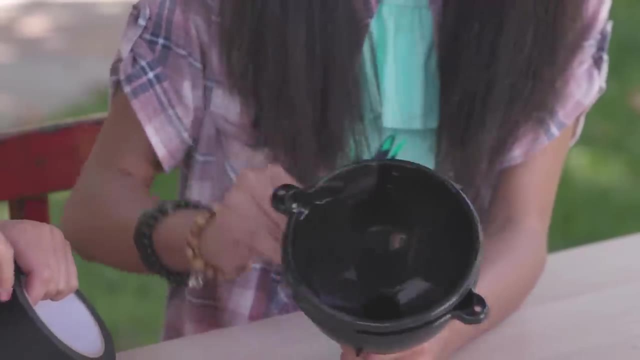 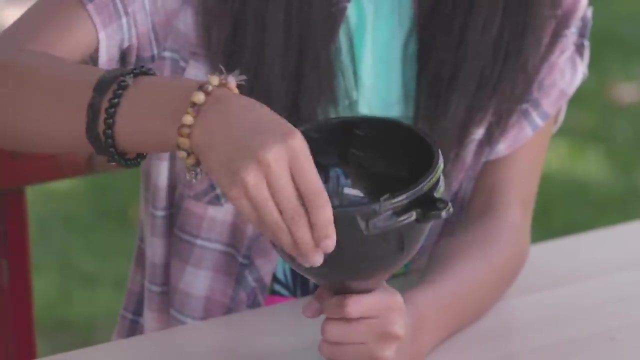 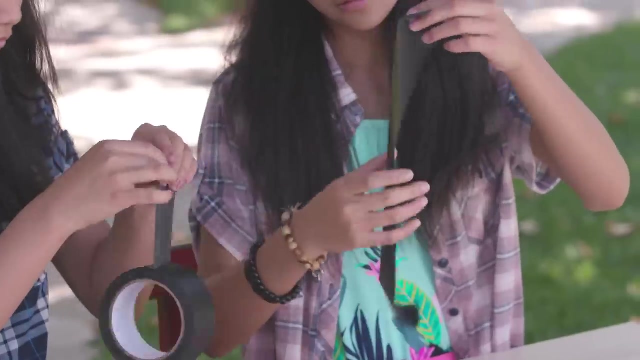 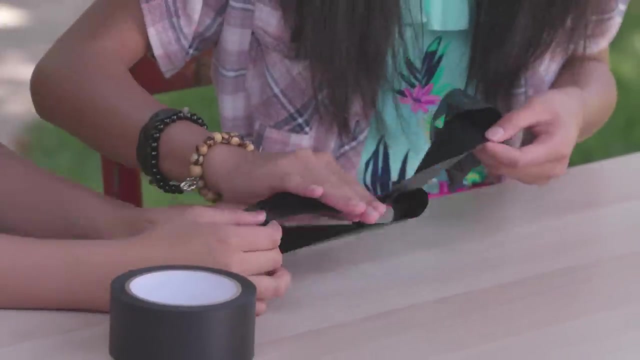 Place one funnel inside the other one so that the holes are across from each other. Secure them together with tape. Make a loop with the tape that's big enough for your hand to fit inside of. Now put another loop of tape on the outside so that the sticky sides are together. 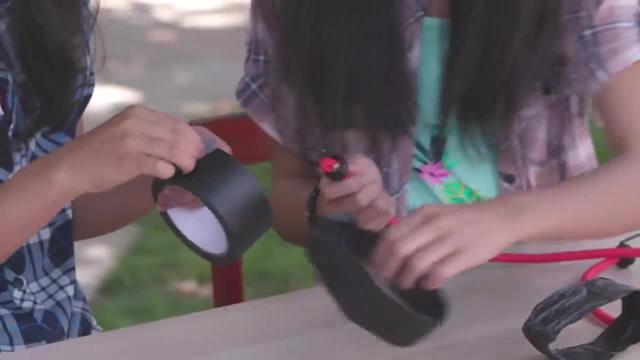 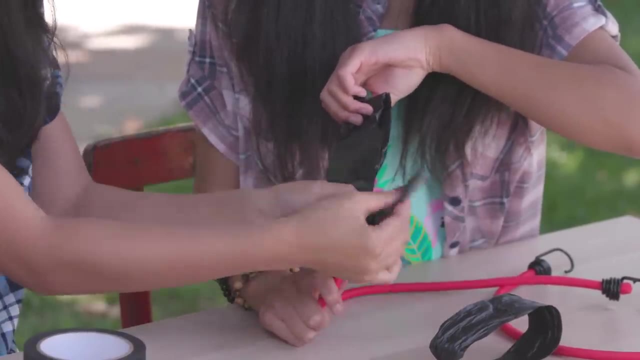 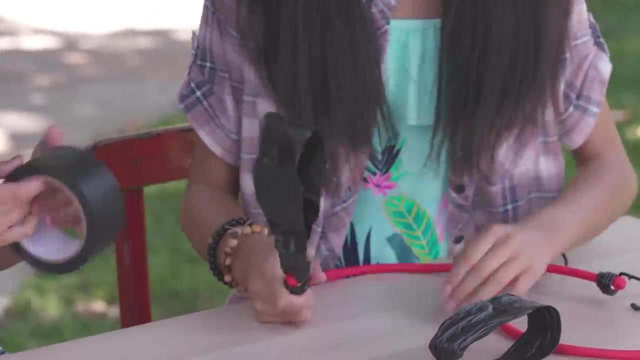 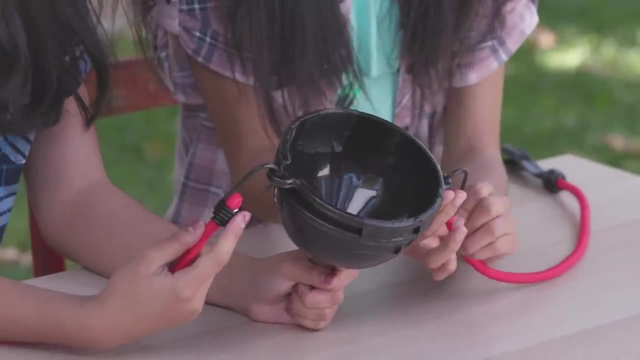 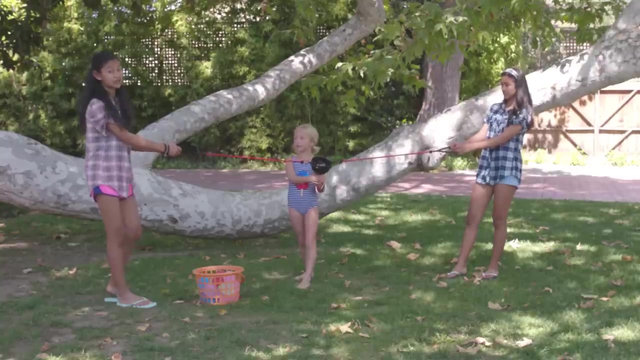 Make two. Put a loop of tape into one hook of the bungee cord and then secure it with more tape. Repeat on the other bungee cord. Now slip the other hooks through the holes in the funnel. To use your slingshot, just have a person hold each handle. 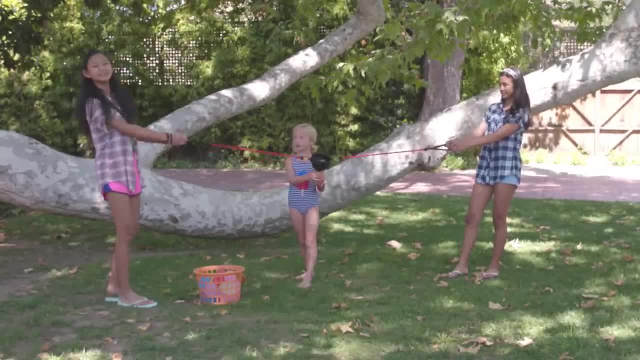 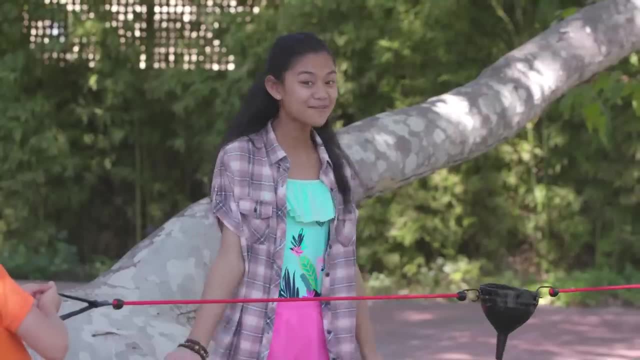 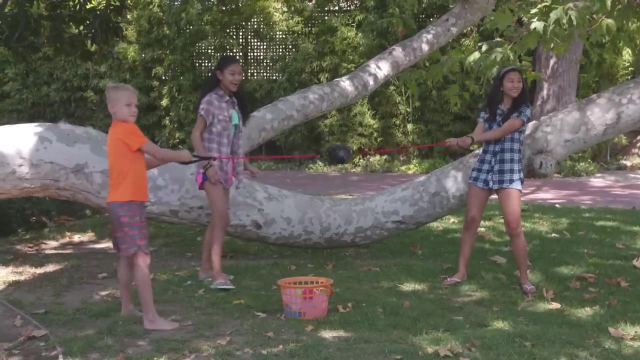 and have another one. pull back the funnel and let the balloon fly. You can aim it at something far away Or something close up. Oh my god, I still wish we had a pool so I can float on water. Well, why didn't you say so You can. 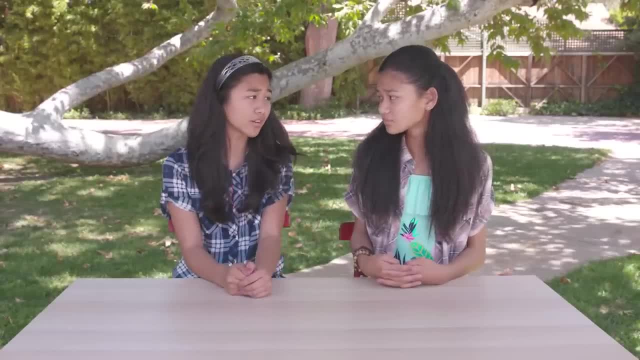 With my DIY water pop. For this hack you'll need a clear shower curtain, parchment, paper, scissors, blue food coloring, duct tape, an ironing board, an iron and a hose. Open up your shower curtain. Open up your shower curtain. 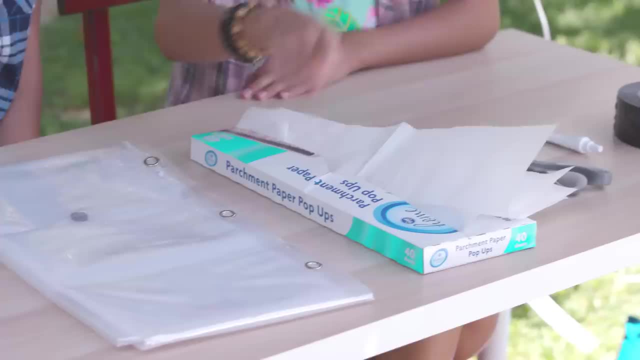 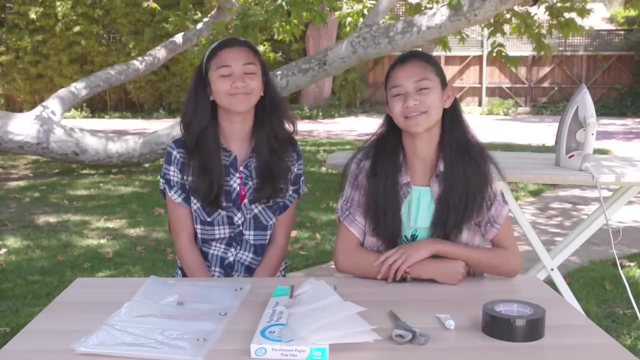 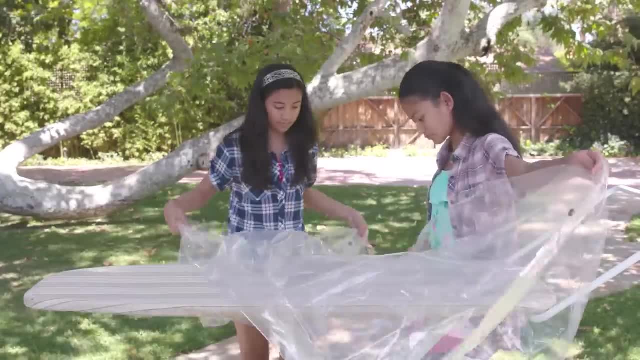 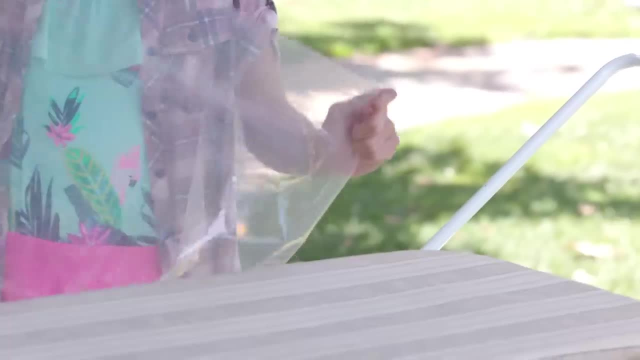 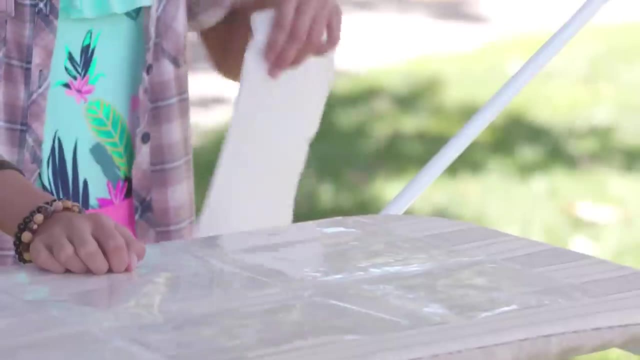 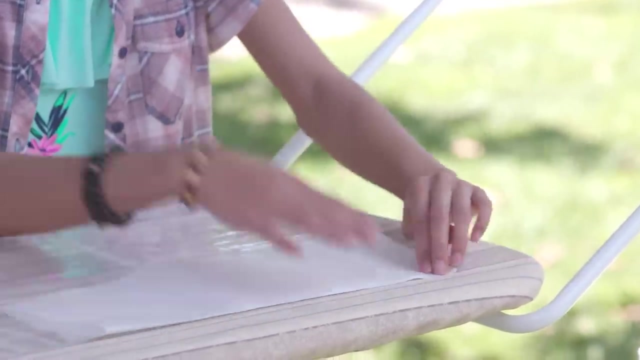 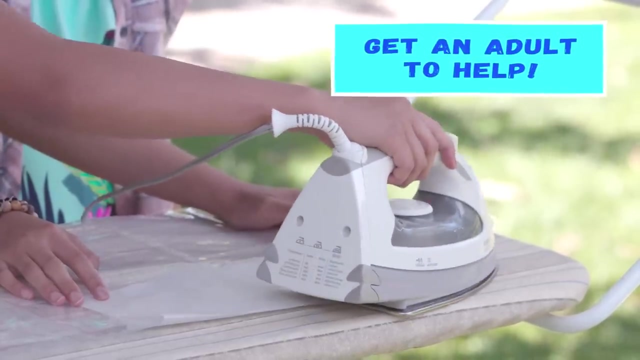 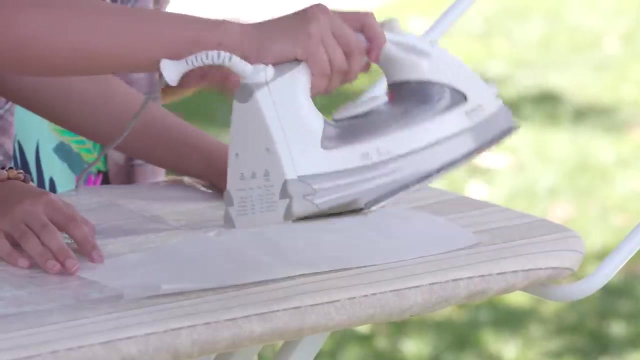 Fold your shower curtain in half. Now lay one edge onto the ironing board, Place parchment paper around the edge of your shower curtain And then use an iron on medium heat to melt the two edges together. Remember to only let the iron touch the parchment paper. 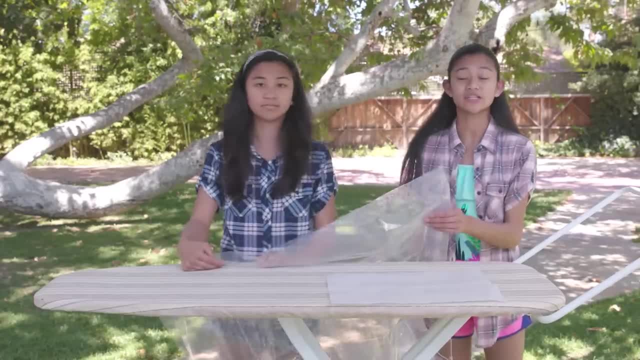 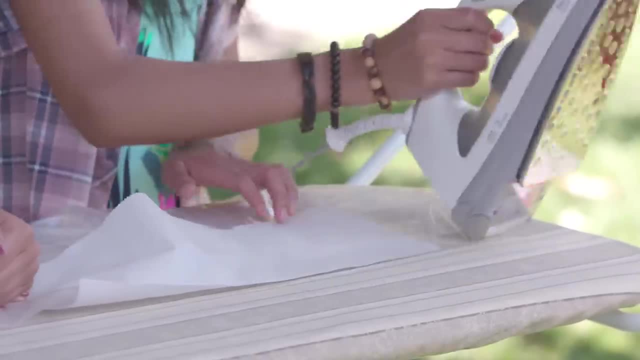 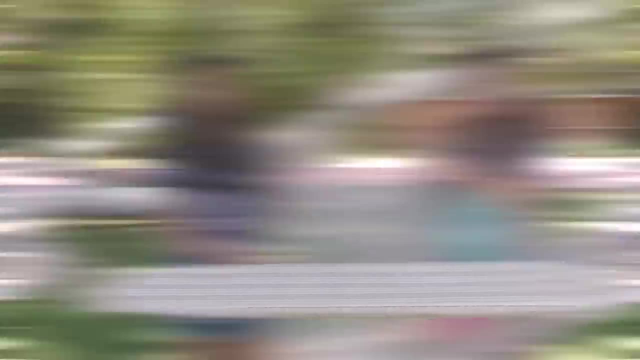 See, the edges are melted together. Now continue this all the way around until you have about three inches of open space. See, we went all the way around the outside and only left a tiny little hole for the hose. Lay your blob down on a place. 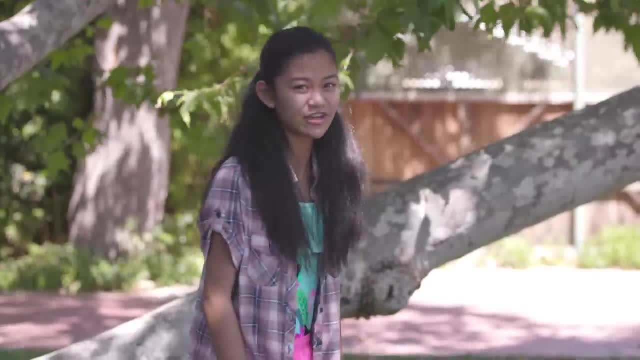 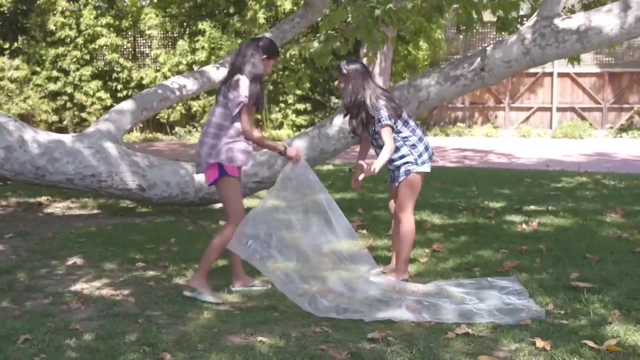 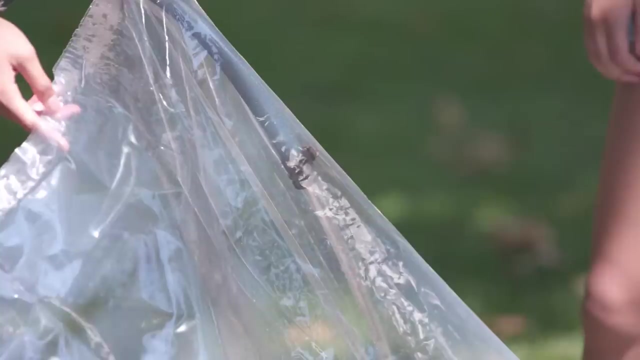 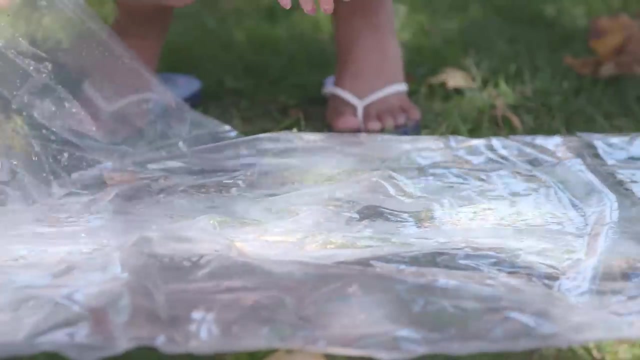 where you want to play with it, because once you fill it with water it could be a little heavy, And then use the hose to stick it inside that tiny hole you made and then fill it up. When it's about halfway full, add a good squirt of food coloring.